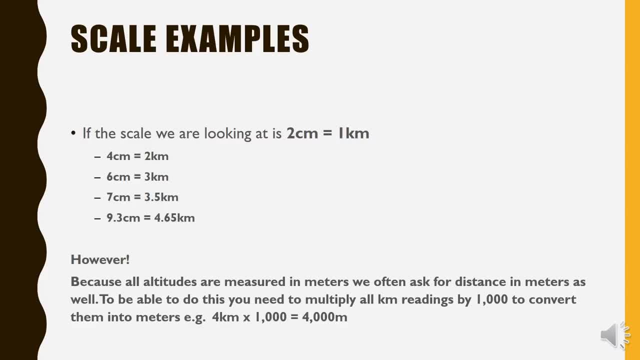 equal 2 kilometers, 6 centimeters, 3 kilometers, And you can even go more precise. So if you are 3.9 centimeters, this could equate to 4.65 kilometers. It is, however, very typical that you will be asked to calculate a distance not in kilometers but in meters. This is often done. 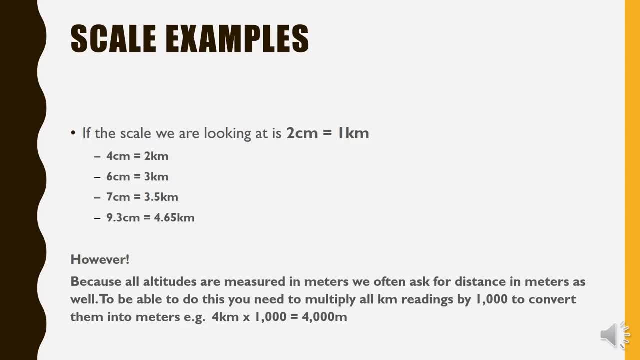 when we want to keep the units the same and we measure altitude always in meters. To be able to do this, you need to remember that 1 kilometer equals a thousand meters, and then you multiply whatever your reading is by the thousand meters. For example, 4 kilometers times a thousand would. 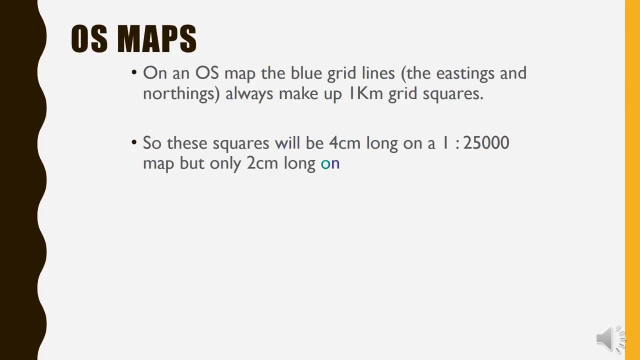 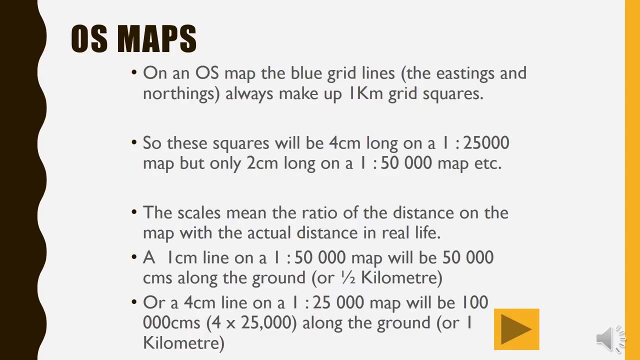 be 4,000 meters. Before we jump in and look at real life examples of how to calculate distance on the map, I just want to quickly summarize. So, on alternate survey maps, the grid references or the blue lines that separate out sections and create squares, These always measure one kilometer. 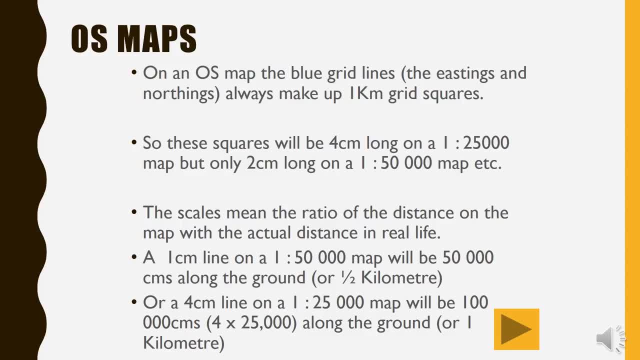 each And the squares will be 4 centimeters long on a 1 to 25,000 scale or 2 centimeters long on a 1 to 50,000 map. The scales mean the ratio of the distance on the map of the actual distance in real. 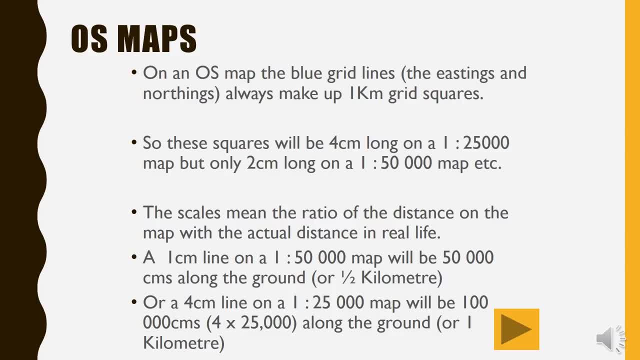 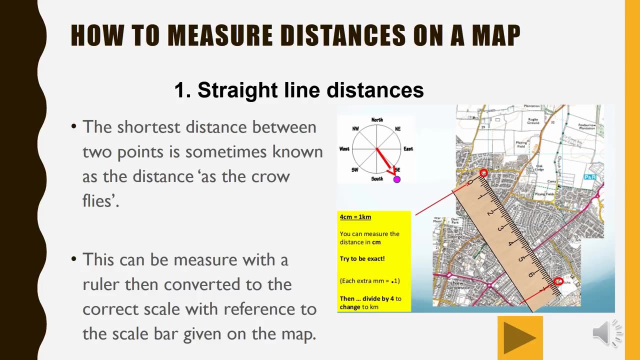 life. Remember, the scale is showing you what it is on the map and you have to use whatever the scale says at the bottom to convert it into real life measurements. The first and probably the easiest distance skill that you'll have to do is to calculate a straight. 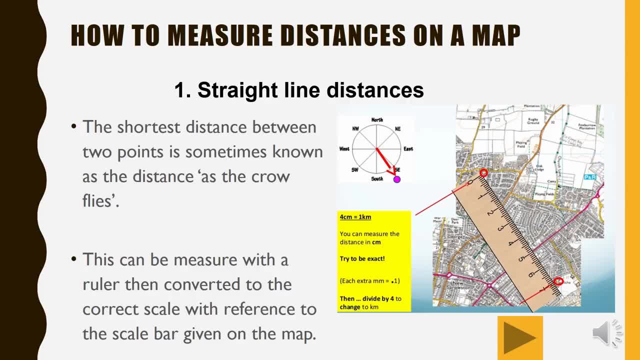 line distance. This is the shortest distance between two points and it's often called as the crow flies, because it basically indicates that a bird or a bird is flying in a straight line. A bird or a crow would fly from point A to point B without deviating from the course or following. 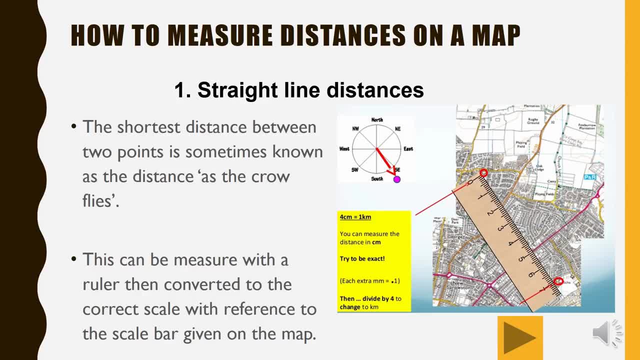 any route. The easiest way to do this is to mark on the map exactly where these two points are, as you can see on the photo, to measure as accurately as you possibly can the distance between these two points, and then use a scale to be able to convert it, As we can see on the image on the right hand. 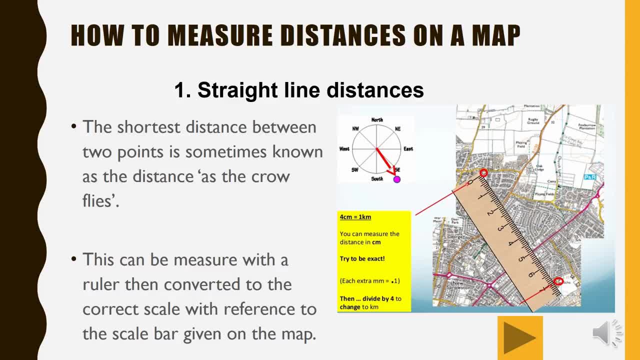 side and we have measured the distance to be around about seven centimeters. So that's about seven centimeters. Therefore, if four centimeters equals one kilometer, seven centimeters is going to be 1.75 kilometers or 1750 meters. 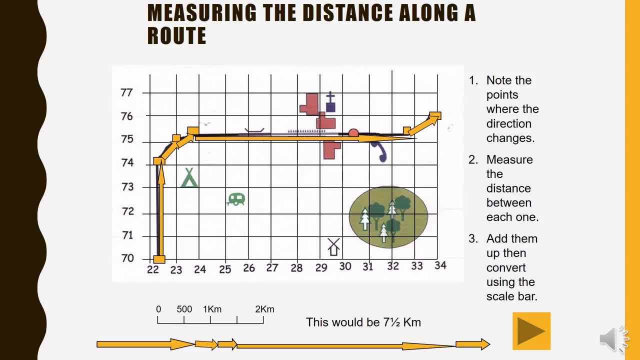 Mething a distance along a route when we don't have an exact straight line is a little bit more complex And, as you can see over here, we have to break down that route into as many straight lines as we possibly can and add them all together to be able to calculate the distance. 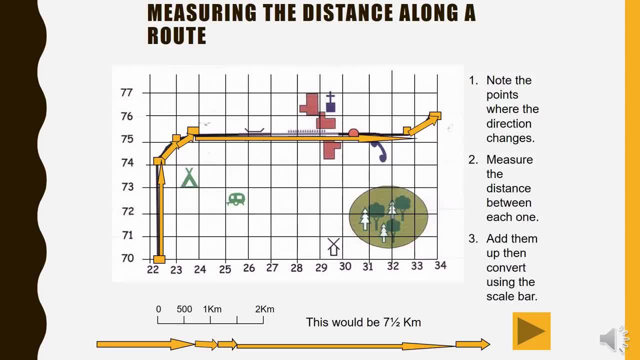 As you can see over here, we've broken down this road- or sorry, I should say our railway track- into our straight lines and we've added them all together, so that way I don't need to go over here at the rack and we can show, therefore, that the distance is seven and a half kilometers. 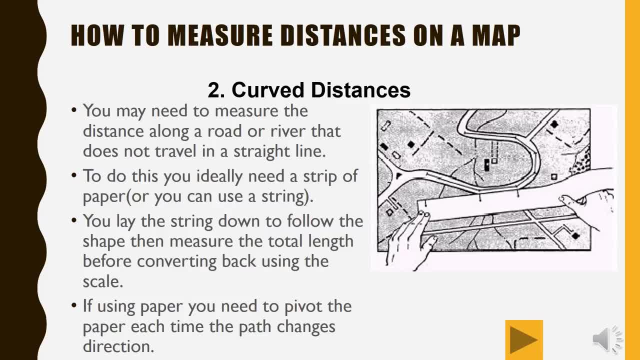 The way that we do this, though, in real life is a little bit more complicated. We need to do this in two ways. You'll need to measure the distance along the road, and you can ideally do this using a strip of paper, or, alternatively, you can use string, and you can just follow the the shape of the road using the. 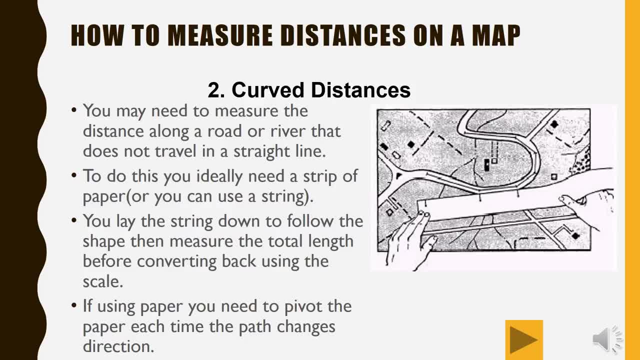 string and then pull it taut. Personally, I prefer using a piece of paper. I find it more accurate, you make less mistakes and I often find that the string is very sometimes hard to manipulate along a complex route. In the following section I'm going to be showing you a video of me calculating and working out a 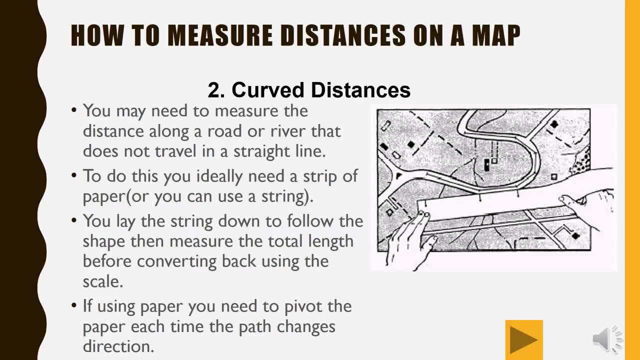 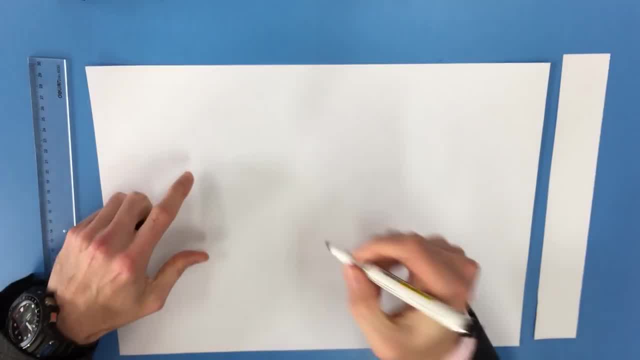 distance along a route using a piece of paper, which is my preferred method. So, as we can see over here, I'm on this piece of paper. I'm going to be marking down two points, A and B, Now the equipment we're going to need to be able. 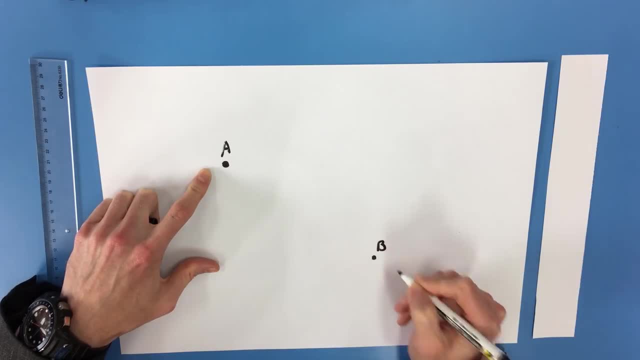 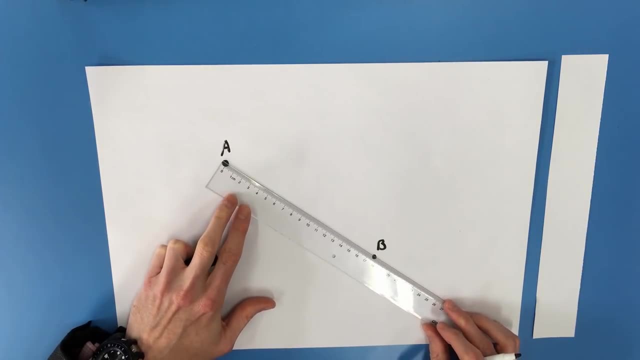 to calculate this distance is a piece of paper that you can see on the right on the screen and the ruler on the left. Now, if there's a straight line distance, it'd be easy. We'd measure A to B exactly as you can see over here. But if we add a, 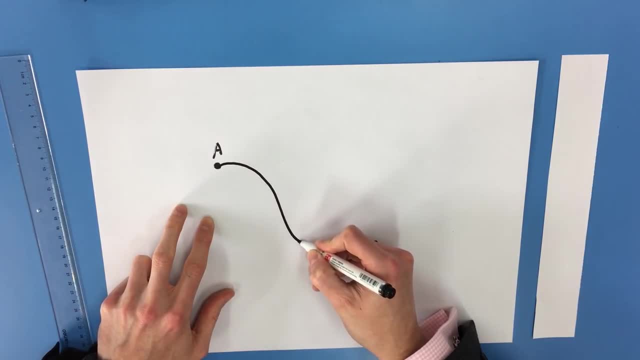 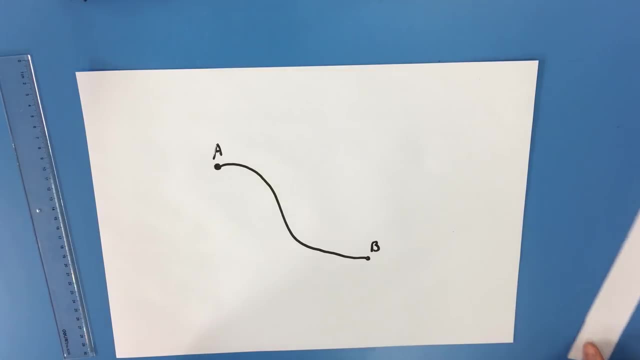 curved line that connects the point A to B. the distance between the two points is A and B, like the one I'm adding now. this becomes increasingly hard To be able to do this. we're going to need to take the piece of paper, The first thing that we. 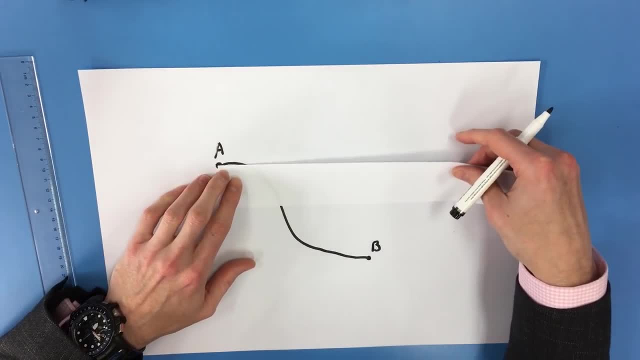 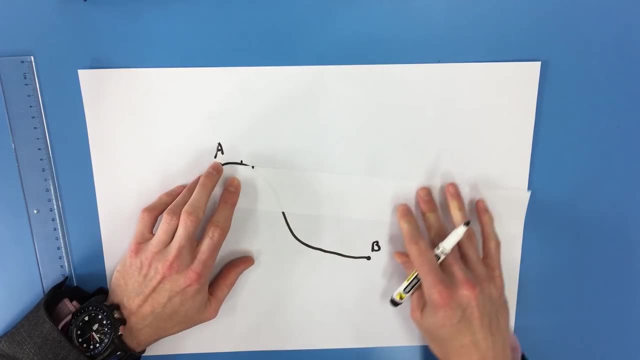 do on this piece of paper is we align one of the corners to the beginning point, the start, and then we try and make some straight lines. As you can see, I'm marking off a straight line there, Then I'm trying to make another straight line. 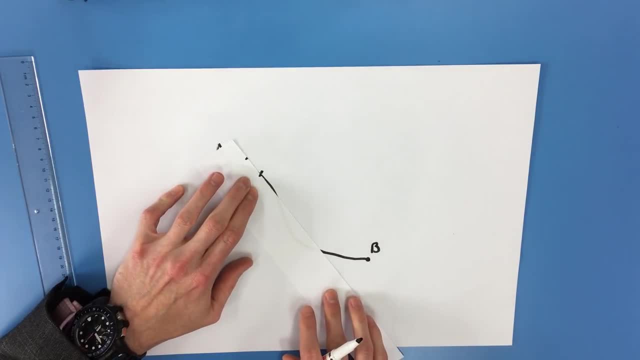 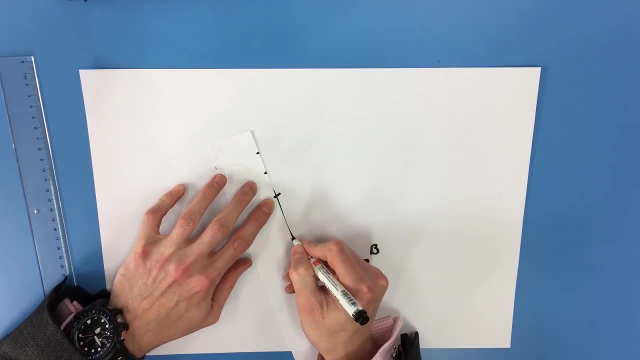 over there And I'll be making a third Now. I keep repeating this until the end. It's very important for you to make a line on both the piece of paper that you're marking and you're measuring and also on the existing map. Now the reason why you do. 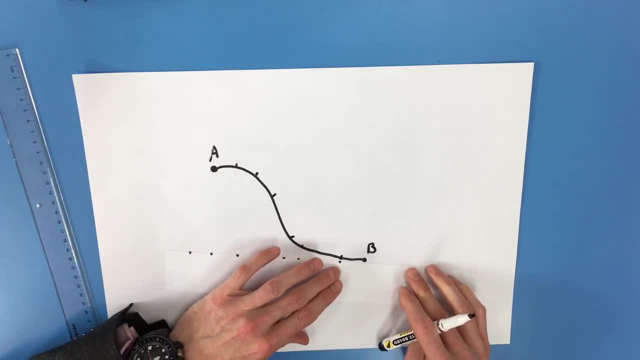 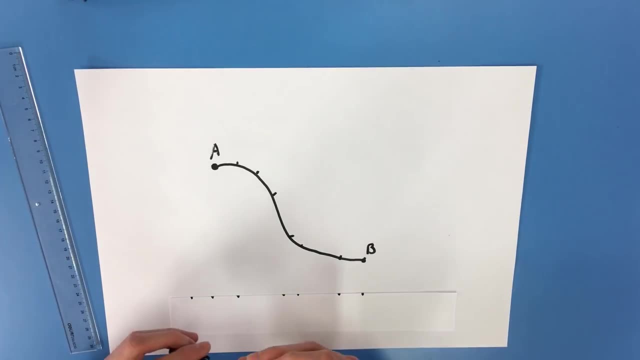 this is to ensure that if, by accident, you move the map, drop the map or lose your place, you can then just realign it with the mark on the map, rather than starting from the beginning After you've made all of your marks on the piece of. 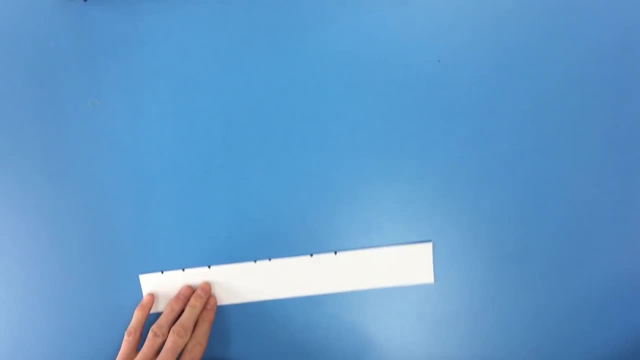 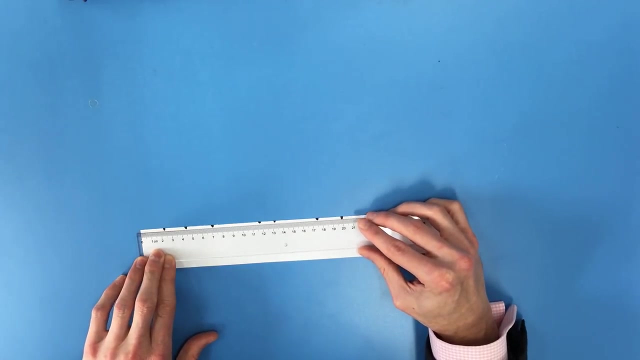 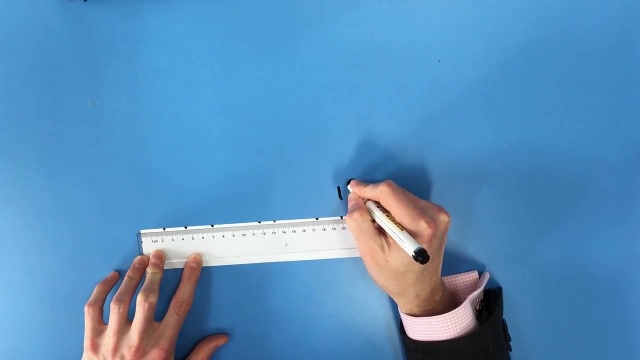 paper. you take your ruler and you measure from the beginning of the piece of paper, the corner that you started, from all the way until the last marked point And as you can see over here- and we've measured the distance and it's going to be 19.9 centimeters distance- We then use 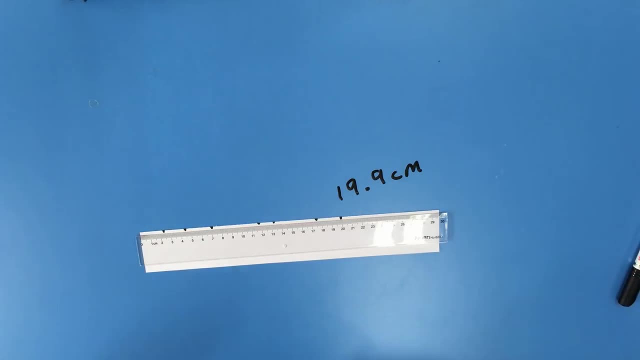 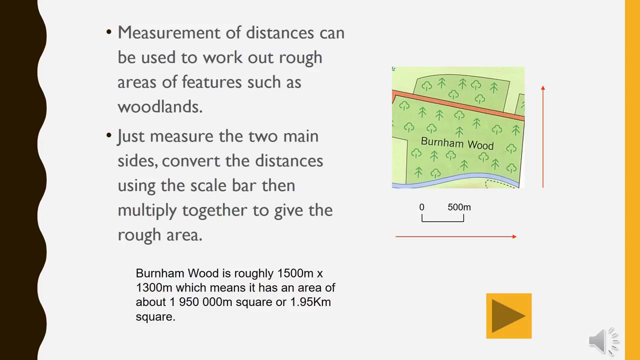 this calculation to be able to find what it is in real life, depending on the scale. Apart from the obvious advantages of being able to work out these distances on the map, being able to calculate how far two places are or to be able to calculate a route from place A to place B distance can also help us calculate. 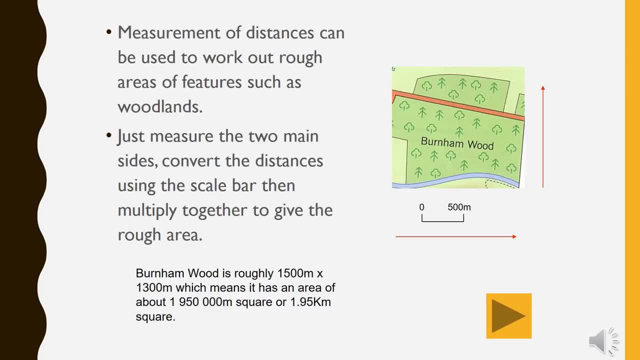 area. We can work out approximate areas on a map. For example, you might be asked to work out the size of a lake, the size of a wood or something like that And, as you can see on this slide, once you've worked out the distance, it's.